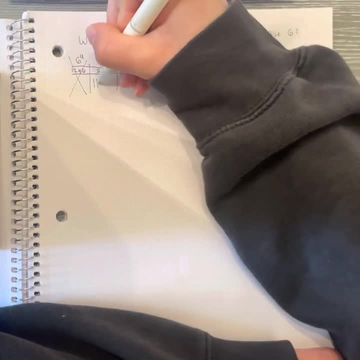 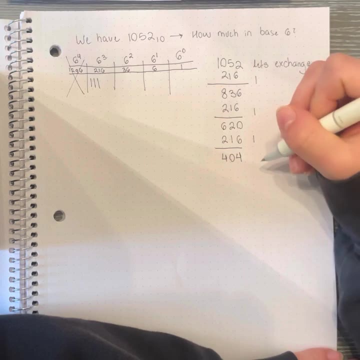 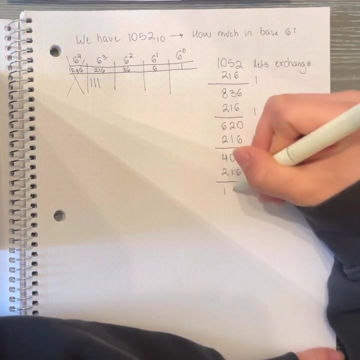 again. so so far we have three. we've exchanged three. okay, now we get four, oh, four, and we just keep going to exchange, so let me get one, he, great. so now that we have one, eight, eight, we can't exchange any more of these, so we have. 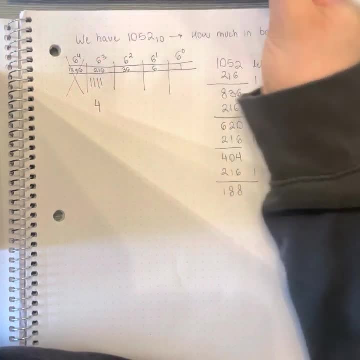 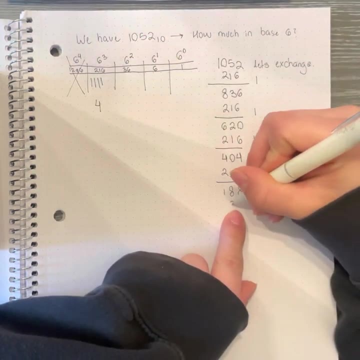 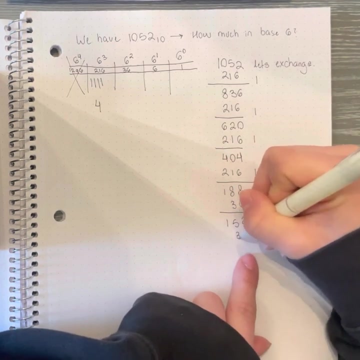 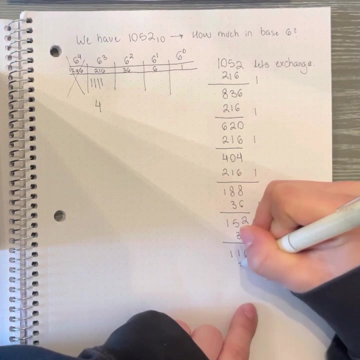 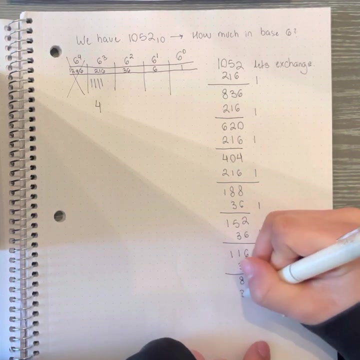 one, two, three, four, boom. so we have four, two, one, six, great, okay. now let's do some thirty sixes, continue exchanging. get one, five, two and then thirty six. one, sixteen, thirty six. we get he six. it's a long process. let me get forty four, okay. eight, okay, now we don't have any more thirty sixes. 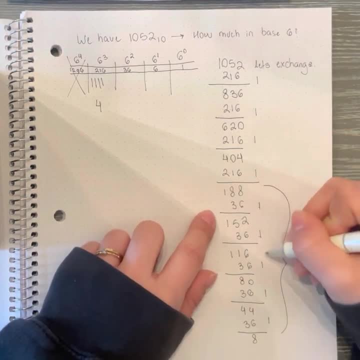 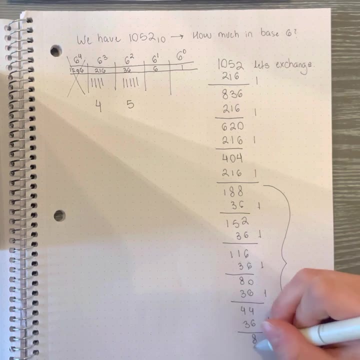 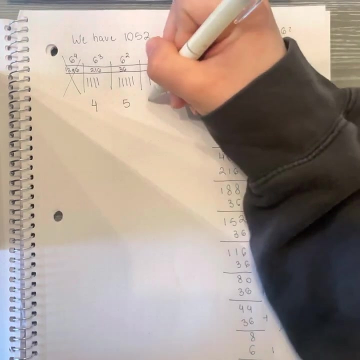 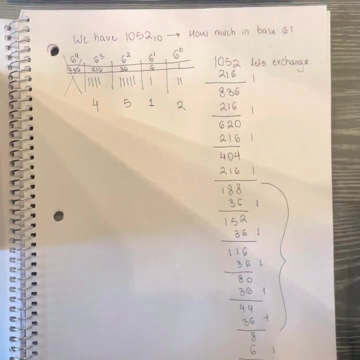 so let me count up these thirty six. I have one, two, three, four, five, great one. two, three, four, five, boom, five. and this one I can only exchange one, six, boom. so I put one six over. here I have one, and then I have two extra great one, two. so this would be our cluster, this is our cups, this is our. 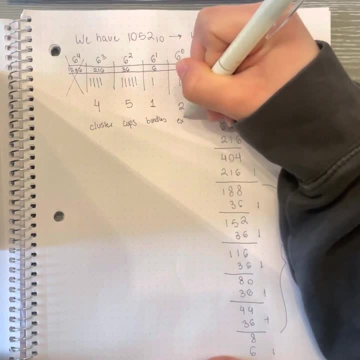 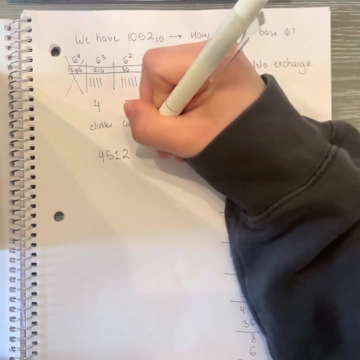 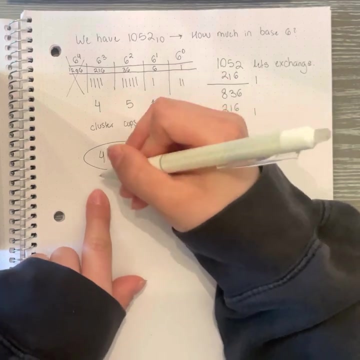 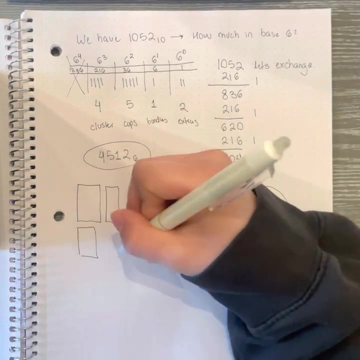 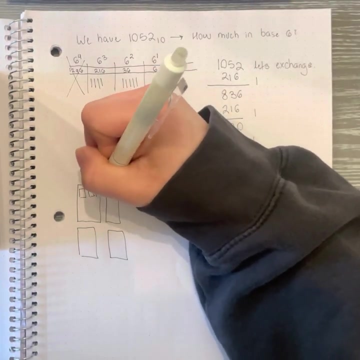 bundles, these are extras, and in total we get four, five, one, two, base six. and the cool thing is that we can even check our work. so you know, if we put four clusters- one, two, three, four- and each cluster has six cups- one, two, three, four, five, six. 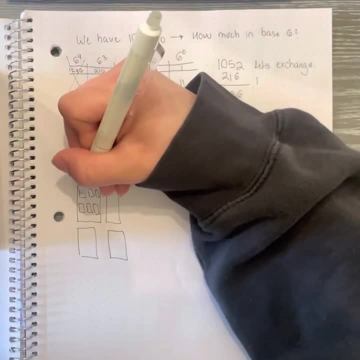 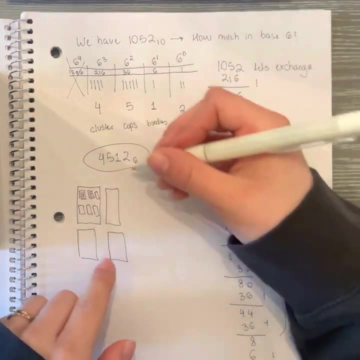 and each of those cups have six, five, six bundles, two, three, four, five, six, two and so on, and then we can check our work by, I guess, like multiplying and one or two times six, you know, and like each cup is gonna have one size, mayim, and each other maybe, but